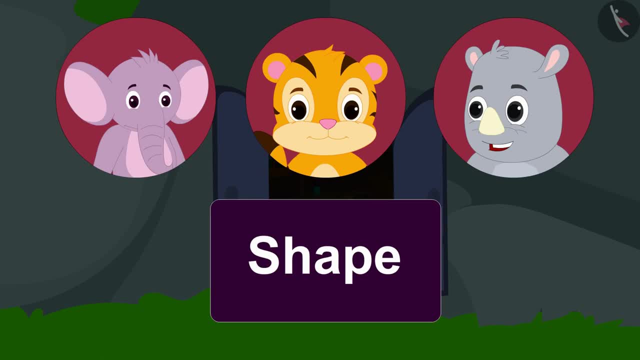 Appu, Sher Khan and Gaggu will look at that shape by turns and come back and make a picture of it. Then the person whose picture most resembles Golu's shape will win First. Appu saw the shape made by Golu. 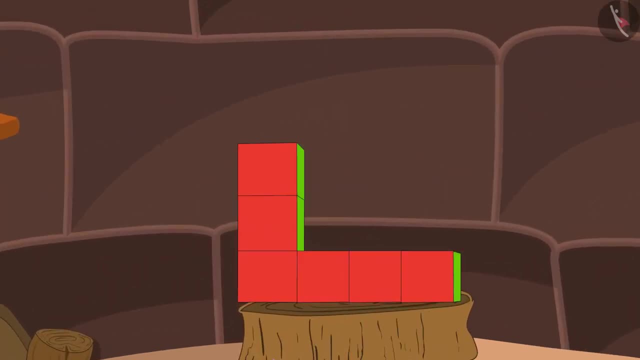 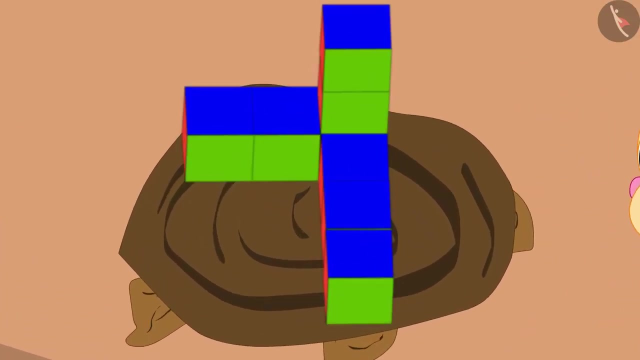 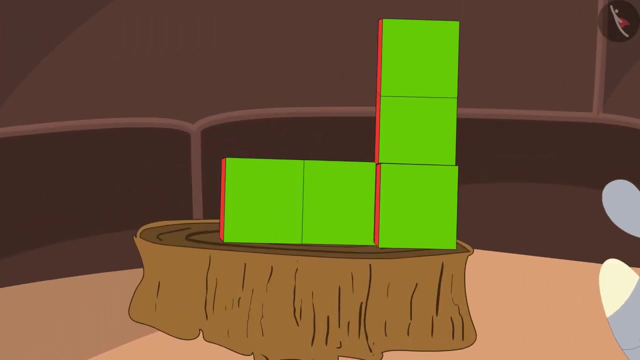 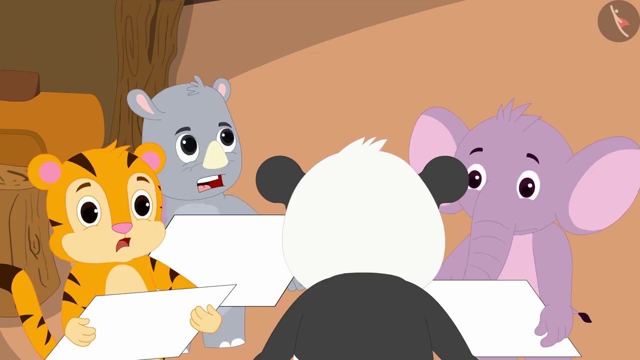 and went and drew his picture. Then Sher Khan also went and saw the shape made by Golu and made his picture. And finally Gaggu went and saw the shape made by Golu and made his picture. All three were shocked when they showed their pictures to Golu. 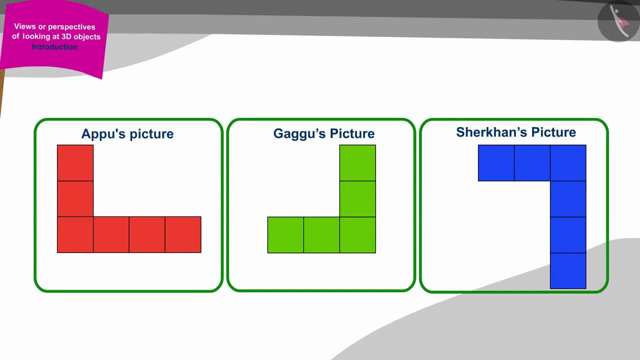 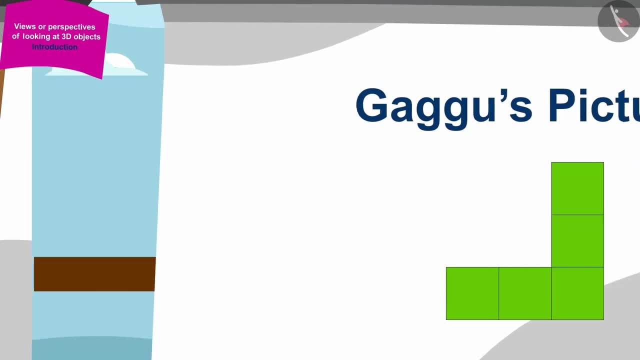 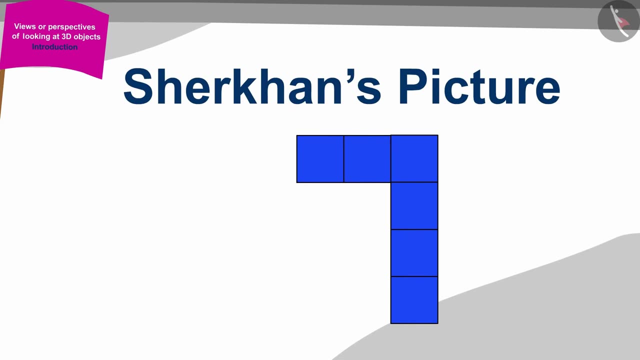 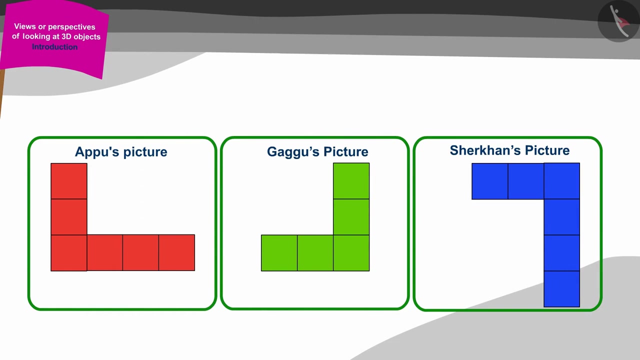 The pictures made by the three of them were completely different. Appu's picture was like this, Gaggu made such a picture, And Sher Khan's picture looked like this. Children, can you tell how this can happen When the three saw the same shape? 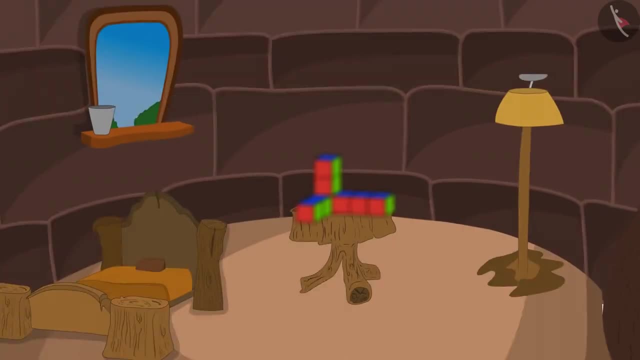 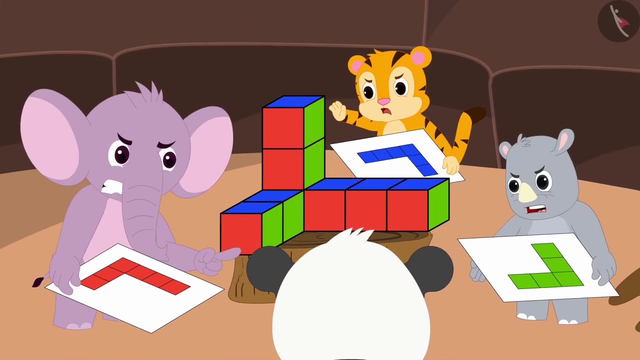 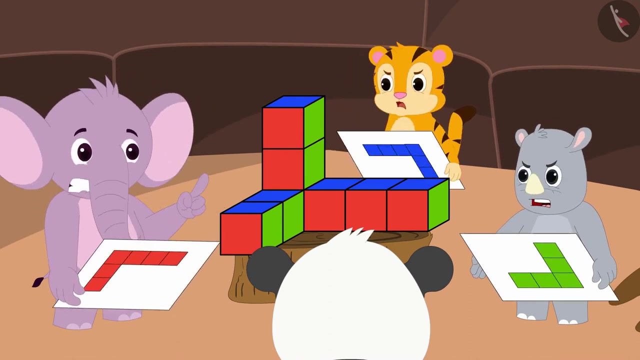 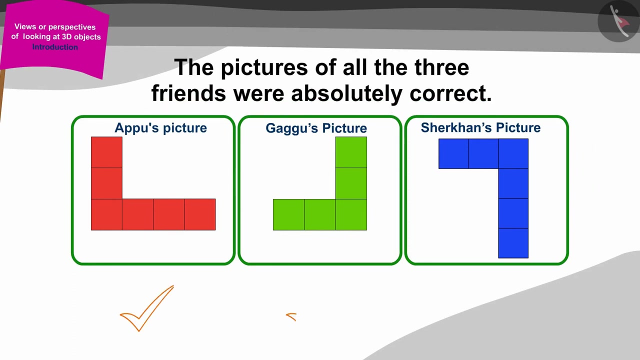 how were their pictures so different? Golu made such a shape out of the boxes. Now the three friends started quarreling about whose picture best matches the shape made by Golu. What do you think is the correct answer? Yes, the pictures of all the three friends are absolutely correct. 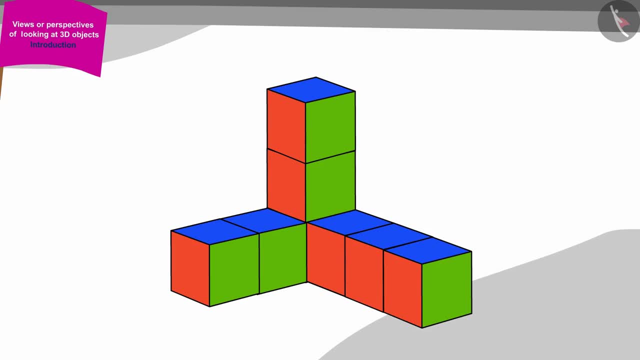 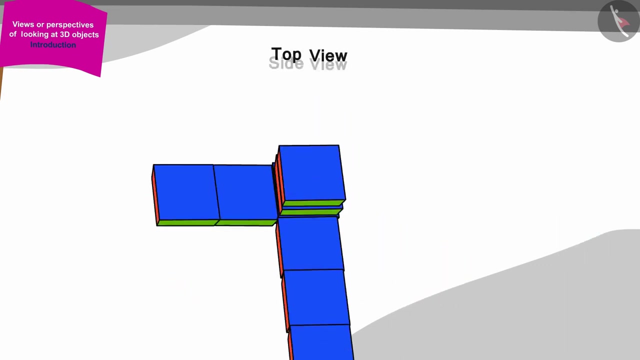 First, Appu saw the shape made by Golu from the front view in this way and made this picture. Gaggu saw the shape from the side view and made such a picture. And finally, Sher Khan saw the shape from the top view. 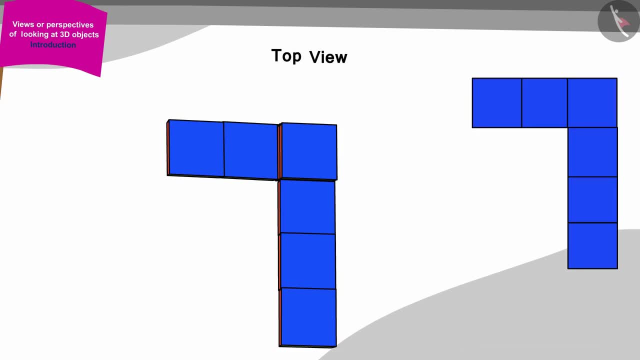 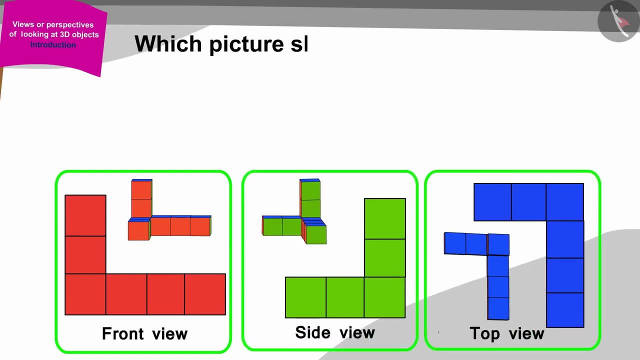 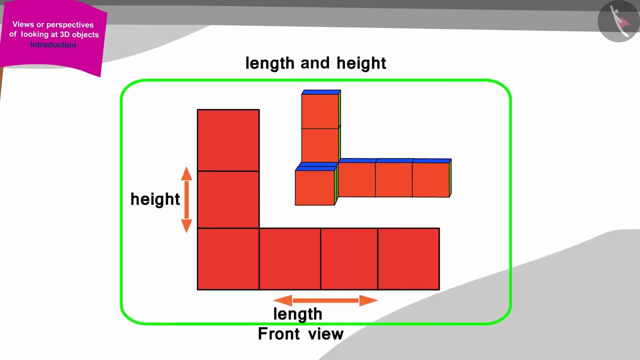 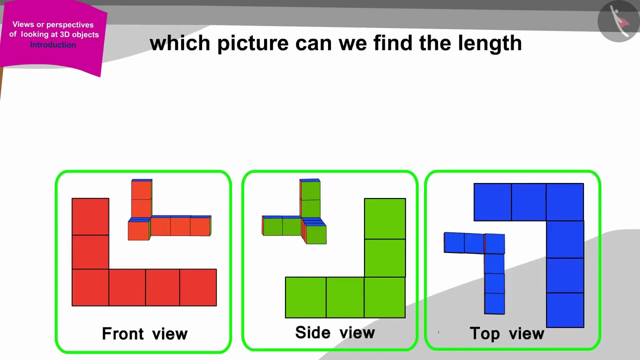 and made such a picture Children. can you tell by looking at which of these pictures you can find out the length and height of Golu's shape? That's correct from this picture, And from which picture can we find the length and breadth?